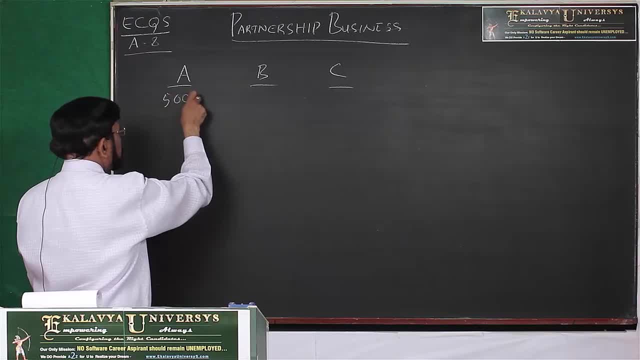 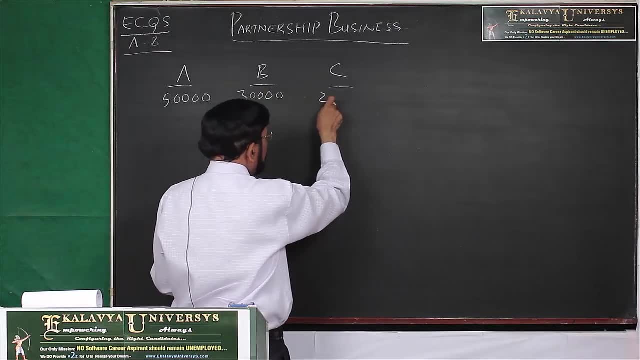 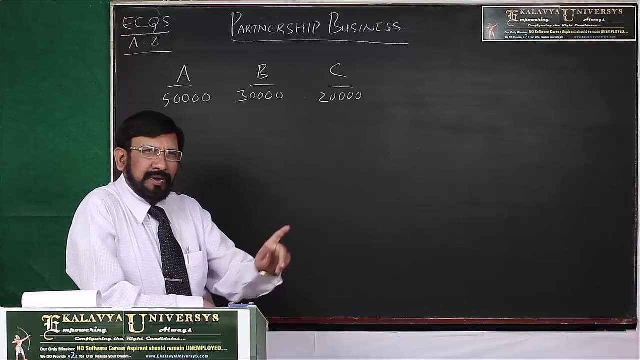 C. A brought 50,000.. B brought 30,000 is as is capital and C brought 20,000, as is capital. Here, earlier I told you one point: They may enter a partnership agreement or they may not. It is not compulsory to enter a partnership agreement. 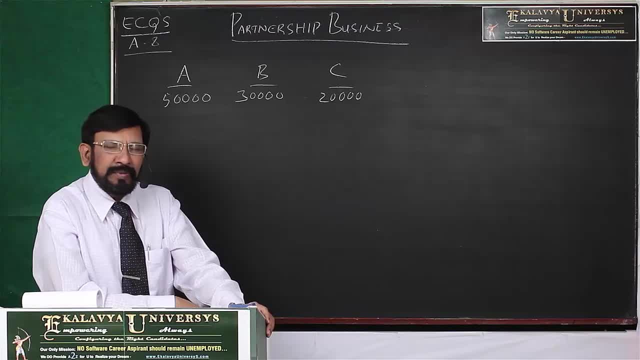 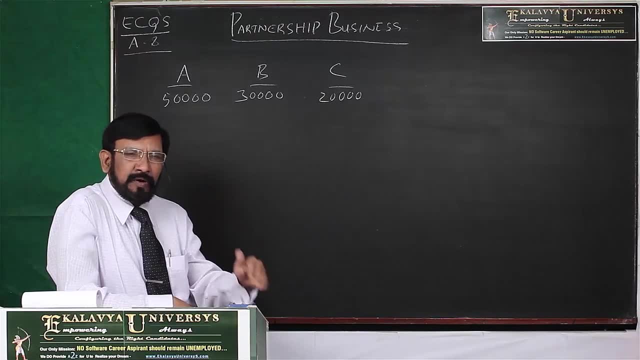 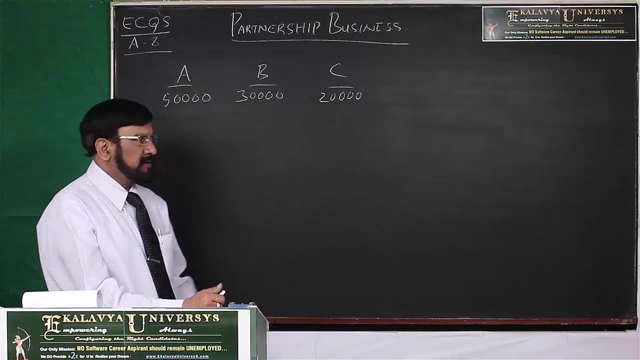 If they enter a partnership agreement through by default, then the hefty amount that they a partnership agreement. in that partnership agreement they should specify in which ratio they are sharing the profits or losses of the business. Suppose partnership, business partnership agreement. specify that they share the profits. 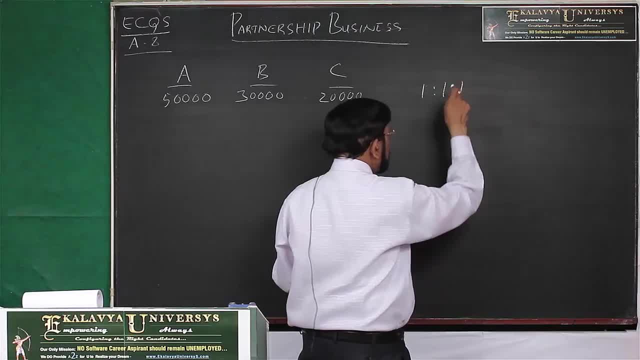 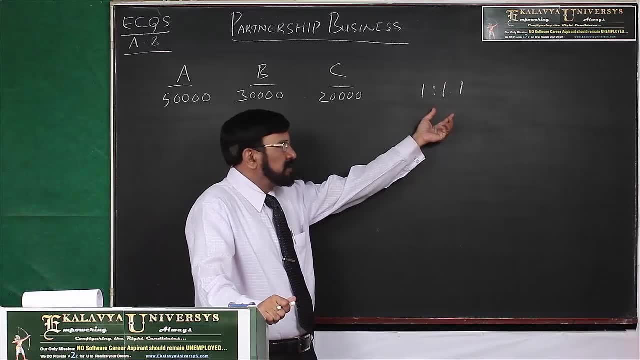 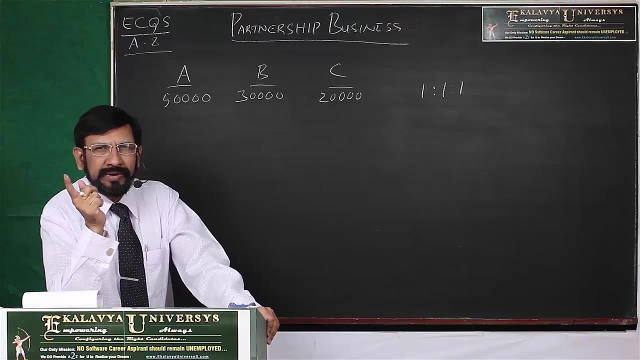 in equal ratio, that is, 1 is to 1 is to 1, then whatever- suppose 30,000 rupees, profits come and all that, they have to share 10,000 rupees each. Just understand this point. if there is any partnership agreement, it specifies the ratio. 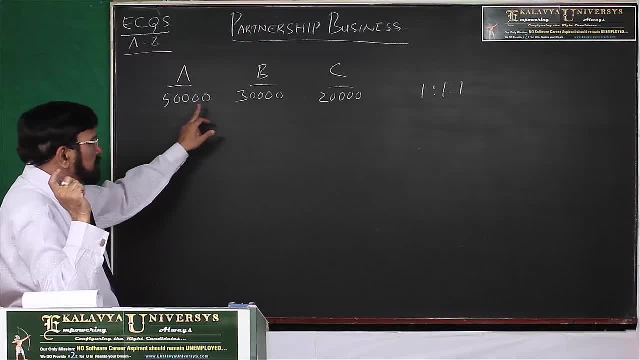 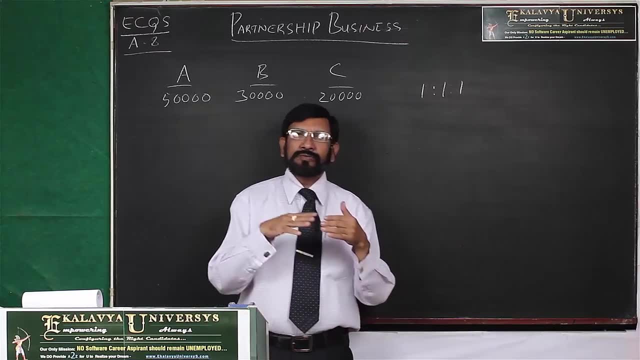 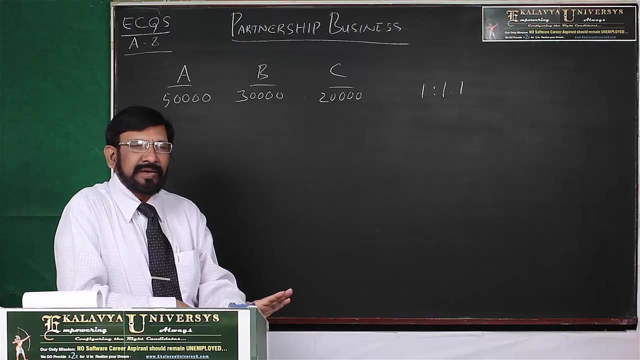 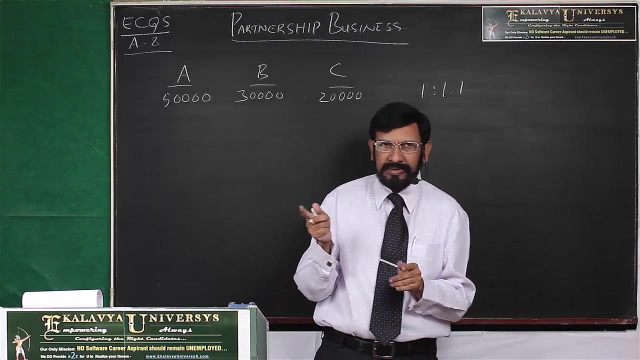 of sharing profits, then, regardless of the capital they brought, they have to share the profits in that ratio. Suppose, if no such agreement is there, it is regulated by the Partnership Act 1932. Then what Partnership Act is telling in case of no partnership agreement is written. 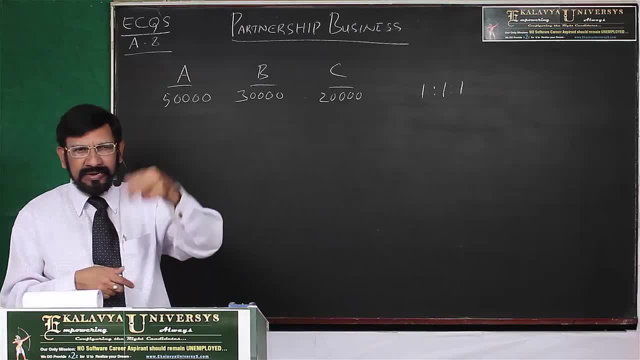 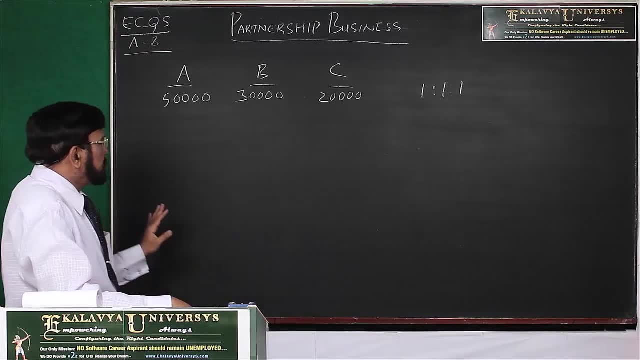 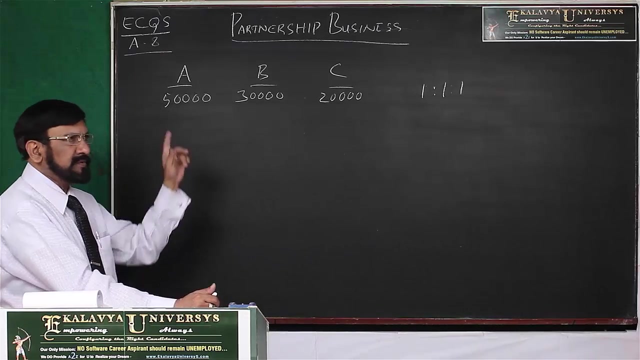 or otherwise, partnership agreement is written. also, if it is silent on the point of sharing of the profits, then in such case they have to share the profits. if no partnership agreement is there or partnership agreement is silent regarding sharing of profits, Then partners should share the profits in the ratio of their capitals. 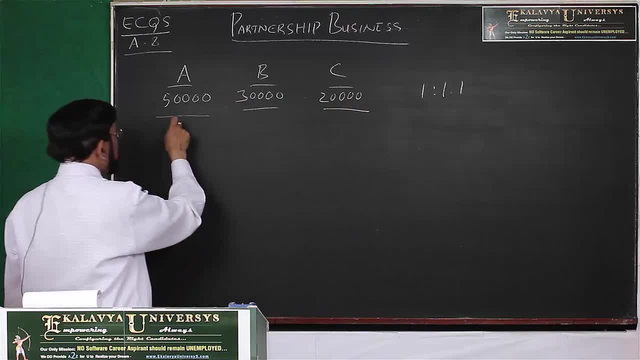 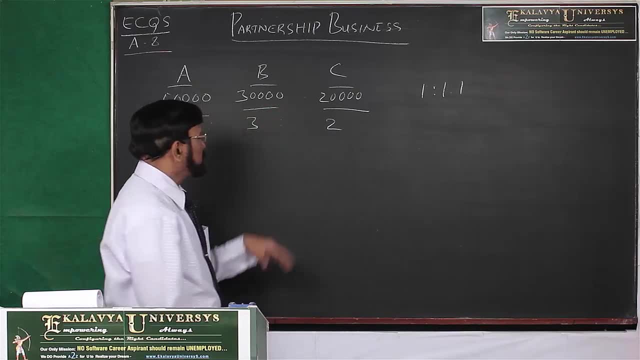 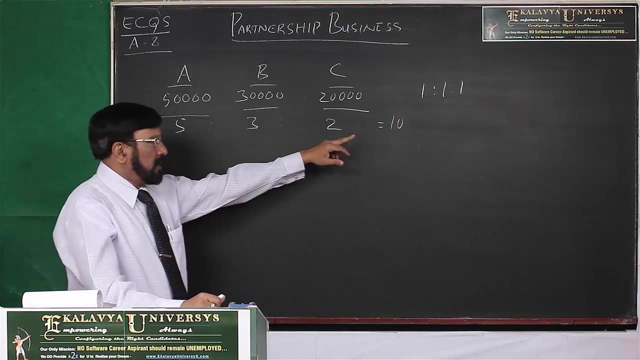 Now let us see their capital ratio. then 5 is to 3, is to 2, now 10,000 goes in everything. 5 is to 3 is to 2, total 10 shares. So if entire profit is divided into 10 shares, then